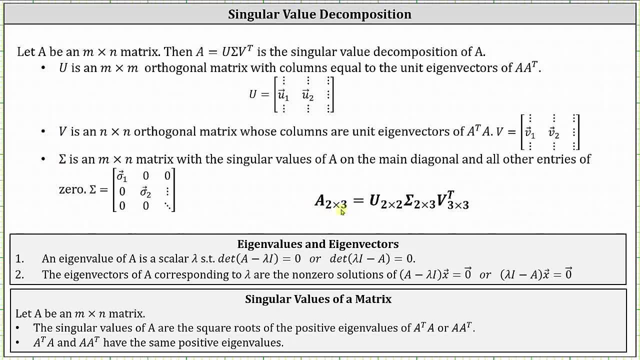 If A is a two by three matrix, m is two and n is three and therefore u is a two by two matrix. sigma is an m by n matrix and therefore sigma is a two by three matrix. and v, transpose, has the same dimensions as matrix v. 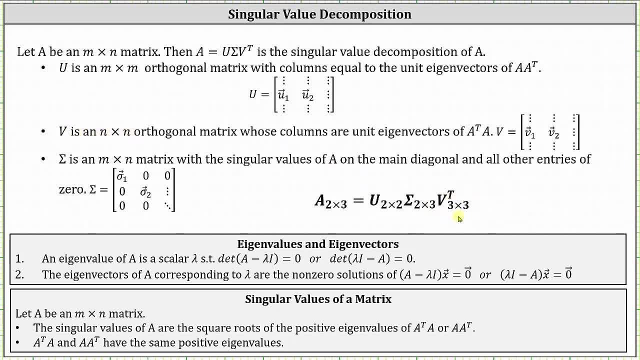 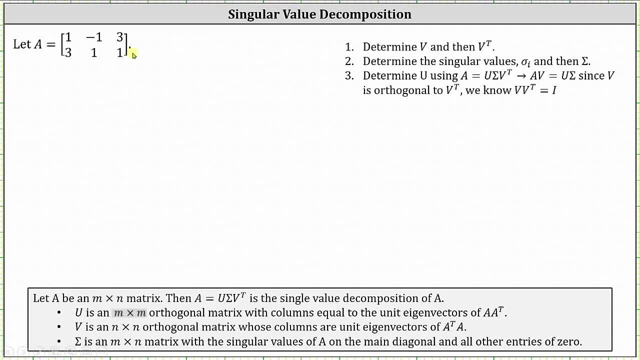 which is an n by n. matrix v transpose is a three by three matrix. And now let's look at an example To find the singular value decomposition of the given matrix. we will follow the three steps shown on the right. Number one will determine matrix v. 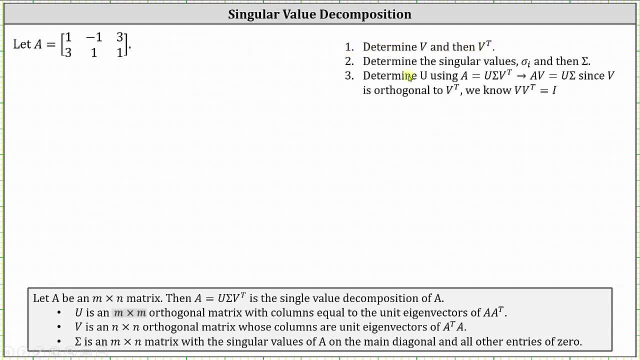 and then the matrix v transpose Number two: we will determine the values of matrix A and then form the matrix sigma, and then step three will determine matrix u by using formulas which we'll discuss more later. So, because matrix v is an n by n orthogonal matrix, 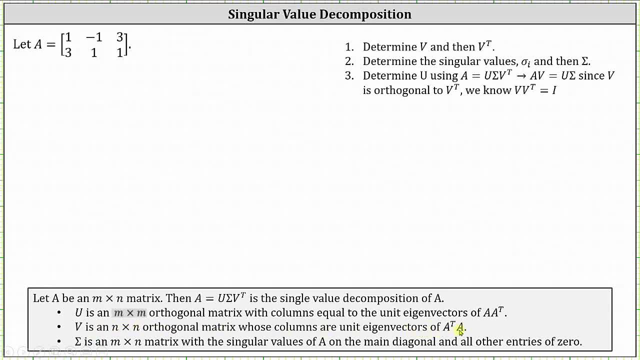 whose columns are unit eigenvectors of A. transpose times A. we'll begin by determining A. transpose times A To find the matrix A. transpose the first row of matrix A becomes the first column of A. transpose the second row of matrix A becomes the second column. 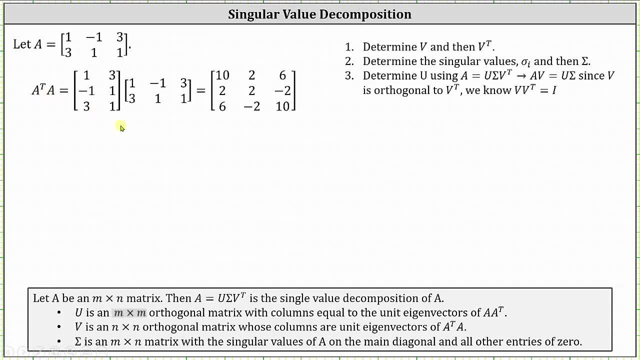 and the third row of matrix A, Wa, is a column of A transpose. A transpose times A results in the three by three matrix shown here on the right. You may want to pause the video and check this product, Because we're looking for unit eigenvectors. 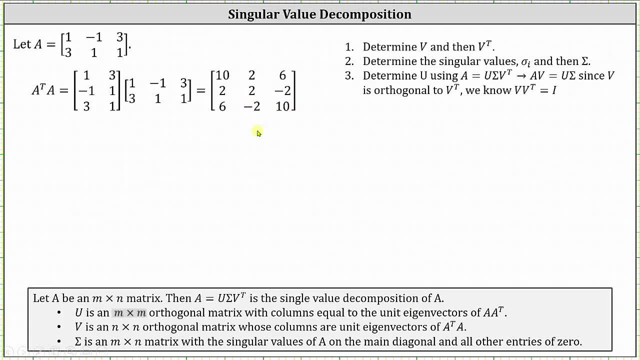 of this three by three matrix. the next step was to determine the eigenvalues. We determine the eigenvalues by solving the equation, the determinant of the difference of matrix A and lambda times. the identity matrix equals zero Where matrix A is a three by three matrix resulting from a transpose times a. 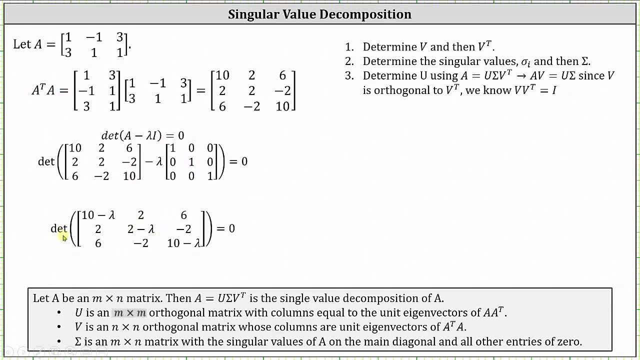 Simplifying inside the parentheses. we now need to find the determinant of this three by three matrix and set it equal to zero. I will go ahead and assume you can find this determinant, which will give us the characteristic equation, The factored form of the characteristic equation. 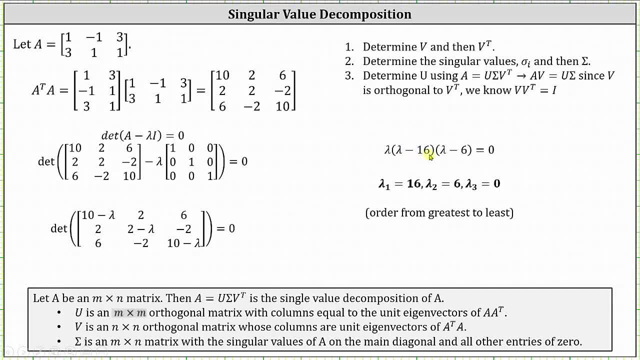 is lambda times the quantity lambda minus 16, times the quantity lambda minus six, which must equal zero. giving the eigenvalues from greatest to least, We have: lambda sub one equals 16, lambda sub two equals six and lambda sub three equals zero. 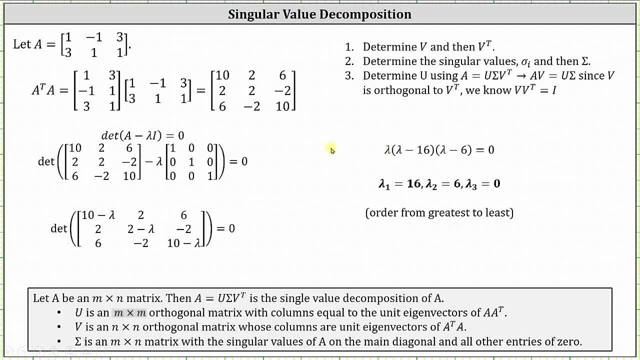 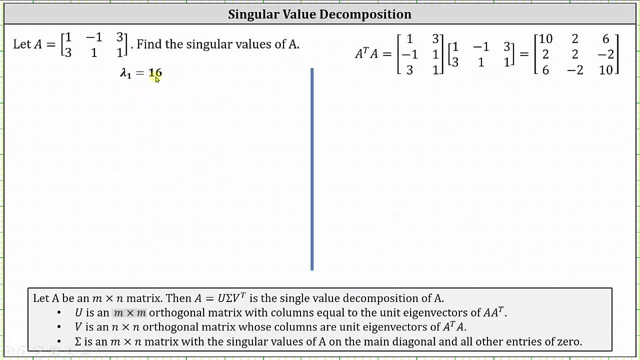 The next step is to find corresponding unit eigenvectors, which will give us the columns of matrix V, and then we can find V transpose, Beginning with lambda, sub one equals 16,. to find the corresponding eigenvectors, we need to solve the vector equation. 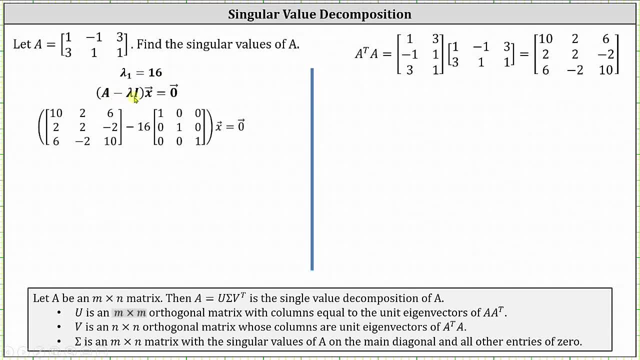 the difference of matrix A and lambda times. the identity of A and lambda is the matrix times. vector x equals the zero vector where vector x is an eigenvector and matrix A is a result of A. transpose times A. I've already set up the vector equation. 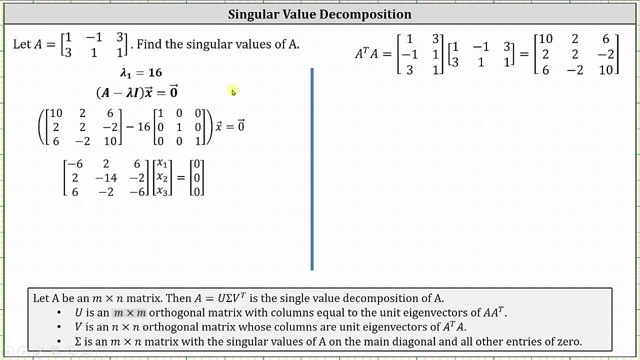 For the next step, we write the matrix equation To find the coefficient matrix. here notice how we subtracted 16 along the main diagonal of the three by three matrix we found by multiplying A, transpose and A. Next we write the augmented matrix. 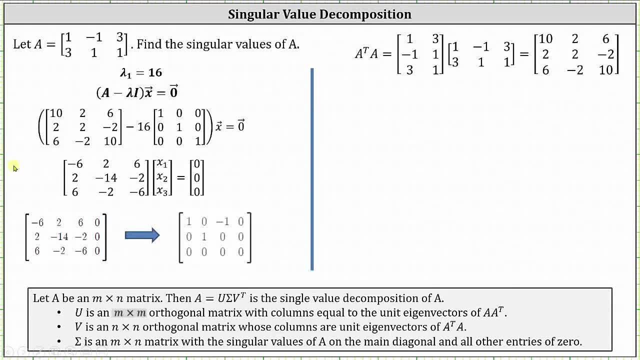 and write the augmented matrix in reduced row echelon form. In reduced row echelon form, notice how the first row indicates x one minus x three equals zero. the second row indicates x two equals zero. x three is a free variable. we have: x three equals x three. 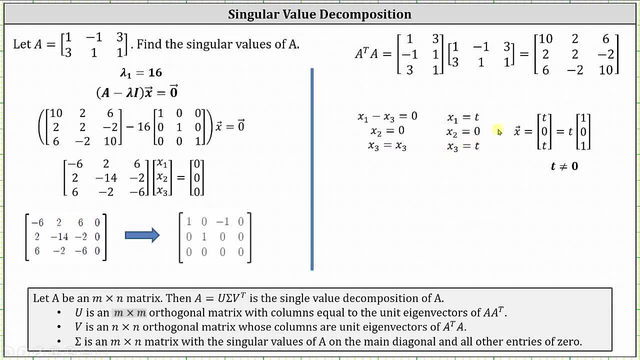 If we let x three equal t, the corresponding eigenvectors are in the form of t times the vector one zero one. If we let t equal one, we would have the eigenvector one zero one, which we need to normalize to find vector v, sub one. 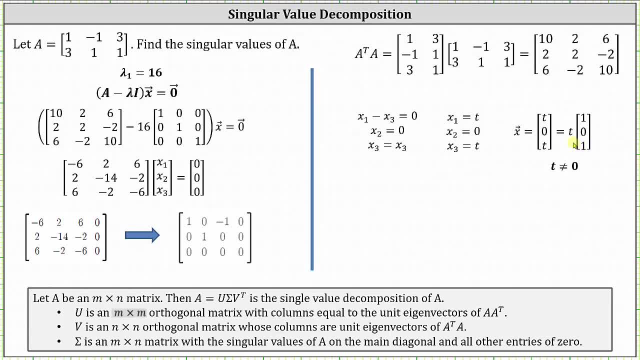 which will be the first column of matrix V. The magnitude of the vector one zero one is the square root of two and therefore the vector v one is equal to the vector with components: one divided by the square root of two zero one divided by the square root of two. 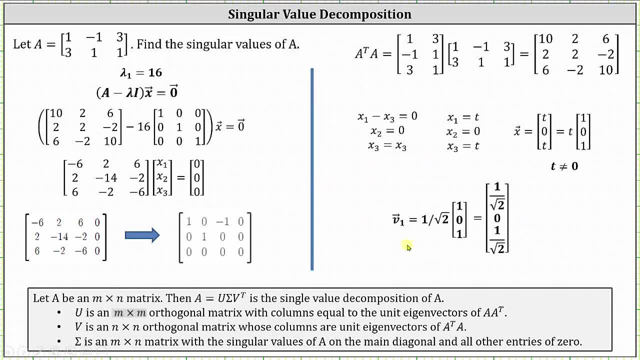 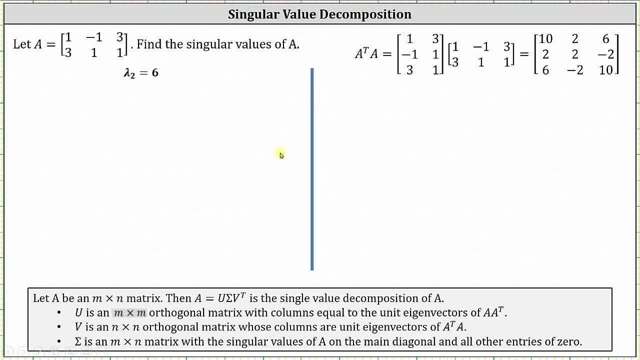 Again, this will be the first column of matrix V. Now we need to go through the same process: for lambda sub two equals six and lambda sub three equals zero. For lambda sub two equals six. we have our vector equation, the matrix equation, the augmented matrix. 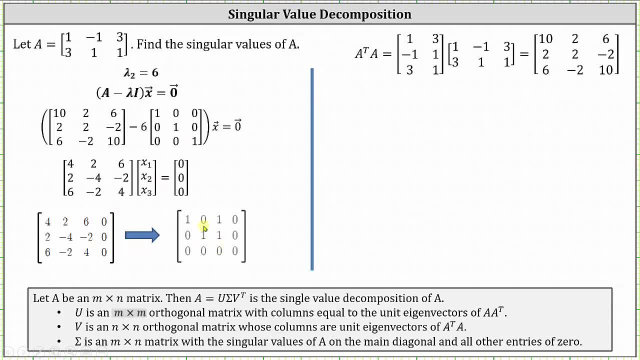 and the augmented matrix in reduced row echelon form. Row one indicates that x one plus x three equals zero. row two indicates x two plus x three equals zero and once again, x three is a free variable, Letting x three equal t the corresponding eigenvectors. 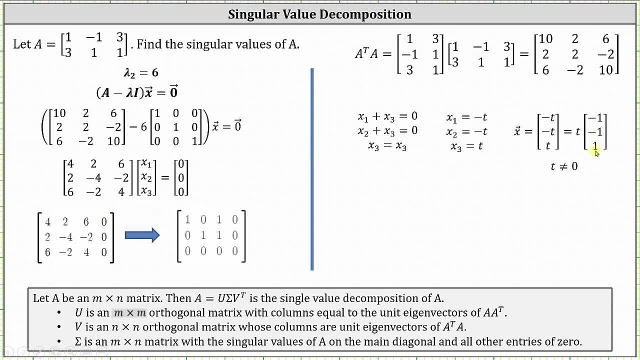 are in the form of t times the vector negative one, negative one, one, again letting t equal one. we have the eigenvector of negative one at negative one, one which we need to normalize to find the vector v sub two, The magnitude of the vector negative one, negative one one. 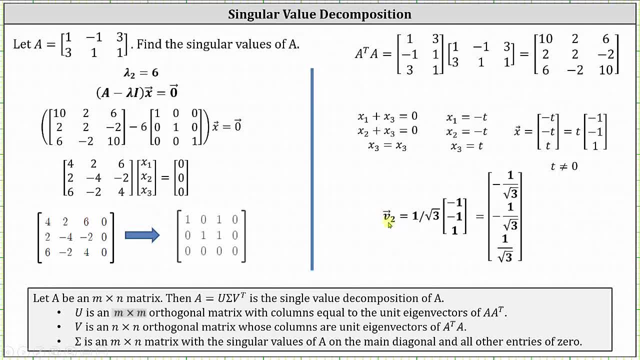 is the square root of three and therefore the vector v sub two, which will be the second column of matrix V, has components: negative, one divided by square root three, negative one divided by square root three and one divided by square root three. 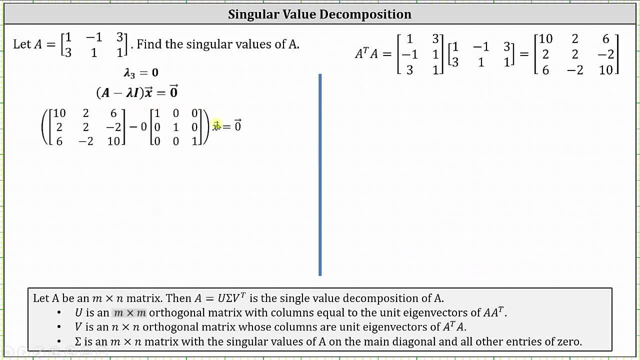 And finally we have lambda sub three equals zero. here we have our vector equation, our matrix equation, the augmented matrix and the augmented matrix in reduced row echelon form. First row indicates x one plus x three equals zero. second row indicates x two minus two x three equals zero. 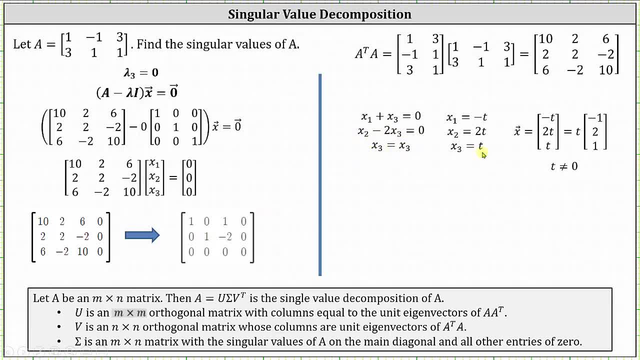 and again. x three is a free variable. Letting x three equal t. we have the corresponding eigenvectors are in the form of t times the vector negative one, two, one again letting t equal one and normalizing the eigenvector. 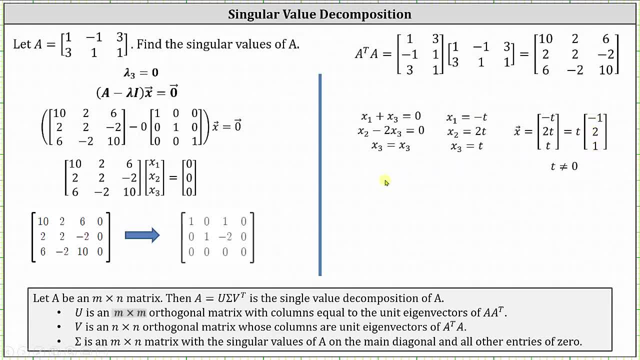 The magnitude of the vector negative: one, two. one is the square root of six and therefore vector v, sub three is the vector with components negative: one divided by square root six, two divided by square root six and one divided by square root six. This will be the third column of matrix V. 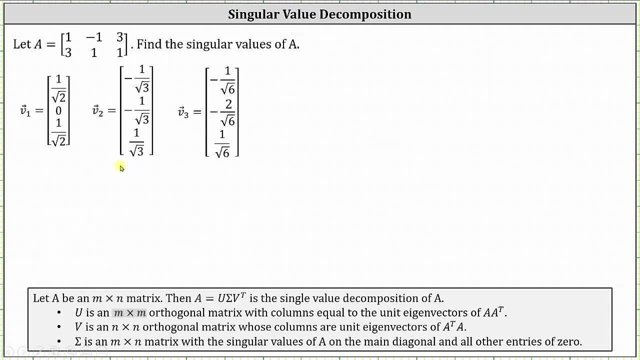 So again, now that we have vector v one, vector v two and vector v three, we can form matrix V where these vectors form the columns of matrix V. and again, for the singular value decomposition, we need v transpose, making the rows of matrix V. 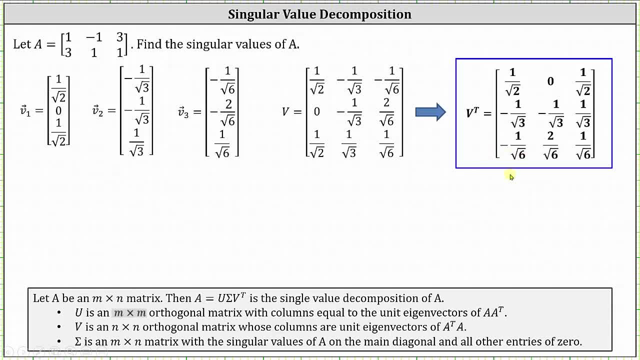 the columns of v transpose. we now have the vector v transpose. Now we'll determine the singular values of matrix A, which will be the entries along the main diagonal of the matrix sigma, and all their entries will be zero. The singular values of matrix A are the square roots. 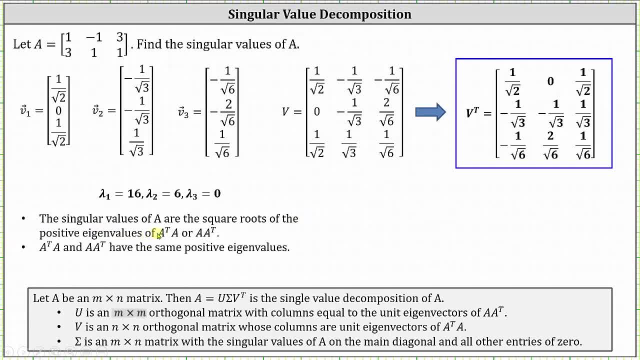 of only the positive eigenvalues of either A transpose times A or A times A transpose. Both of these products have the same positive eigenvalues. Well, we already found the eigenvalues of A transpose times A, which were lambda sub one, lambda sub two. 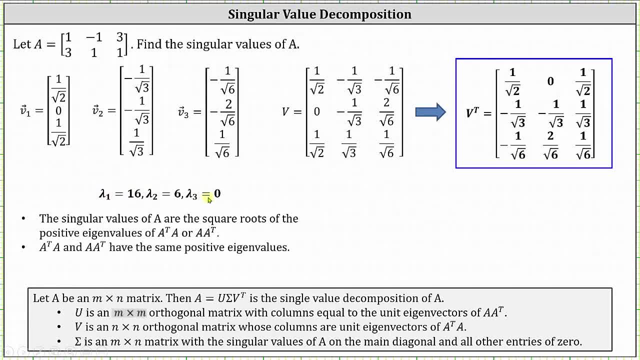 and lambda sub three. We do not include the zero, though. we only use the positive eigenvalues to determine the singular values, And the singular values are equal to the square roots of the positive eigenvalues. We indicate singular values by using the lowercase sigma. 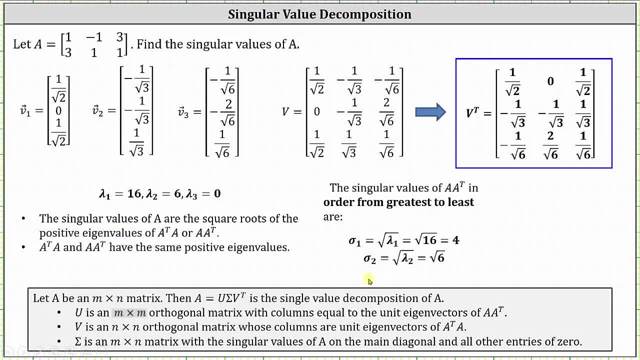 in this case sigma sub one and sigma sub two, which again need to be given in order from greatest to least, And therefore the first singular value, sigma sub one is equal to the square root of lambda sub one, which equals the square root of 16 or four. 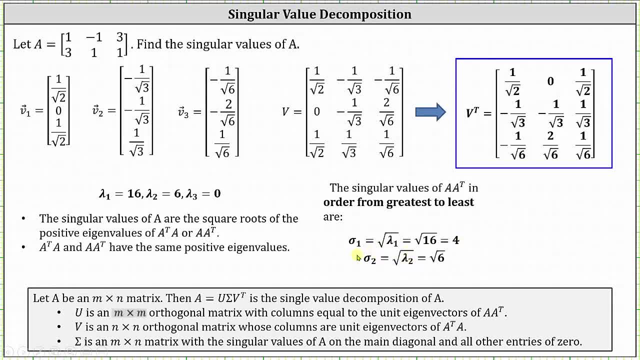 Lambda sub two is equal to the square root of lambda sub two, which equals the square root of six. And now we use these values along the main diagonal of matrix U, which is a two by three matrix, and all their entries are zero. 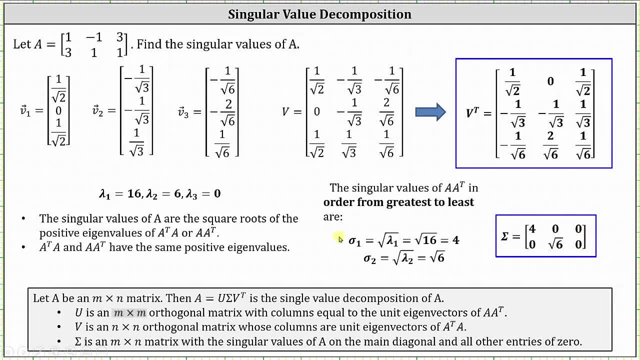 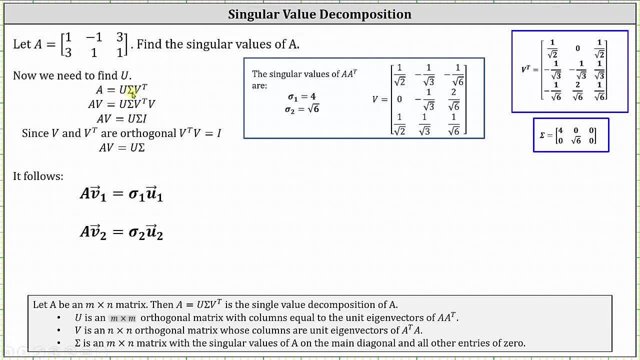 And now we have the matrix sigma. The last step is to find matrix U, which we will do using formulas We know. for the singular value decomposition, we have A equals U times sigma times V transpose. If we take this equation and multiply both sides, 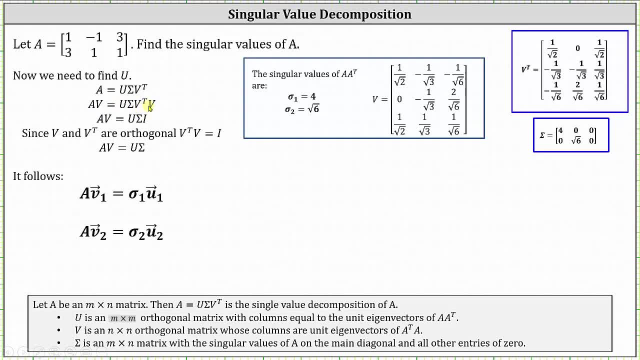 by matrix V. V transpose times V is equal to the identity matrix because V and V transpose are orthogonal, which gives us the equation A times V equals U times sigma, And it works out. it'll give us the formulas below that we can use to find the vector U sub one. 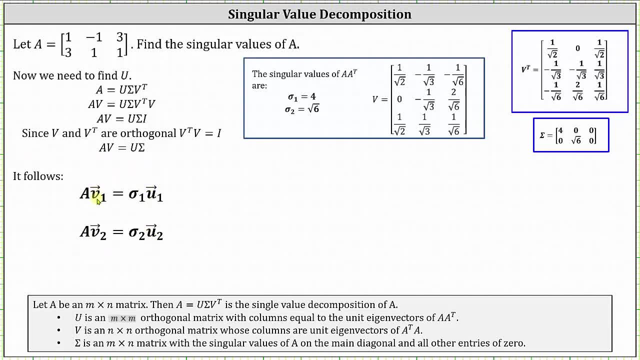 and vector U sub two. It works out that matrix A times the vector V sub one is equal to sigma sub one times the vector U sub one, And similarly, matrix A times vector V sub two is equal to sigma sub two times the vector U sub two. 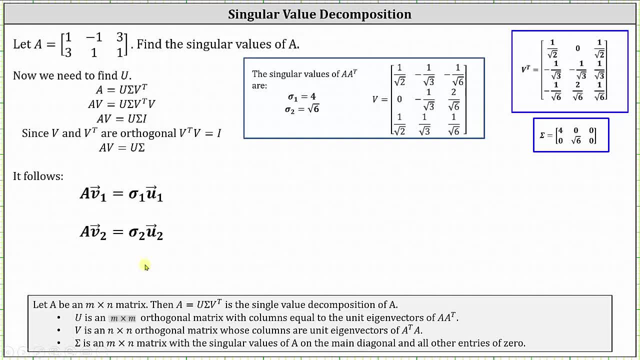 From here we can find vector U sub one and vector U sub two. Solving the first equation for vector U sub one, we would divide both sides by sigma sub one, which gives us vector U sub one equals one divided by sigma sub one times matrix A times the vector V sub one. 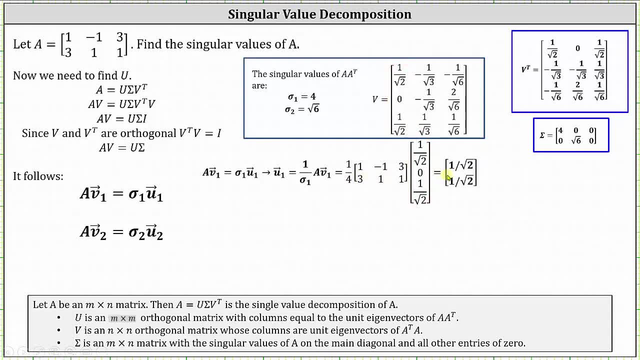 which I've already written out here. The result is the vector U sub one with components one divided by square root two, one divided by square root two. And using the second equation we can solve for vector U sub two. Vector U sub two equals one divided by sigma sub two. 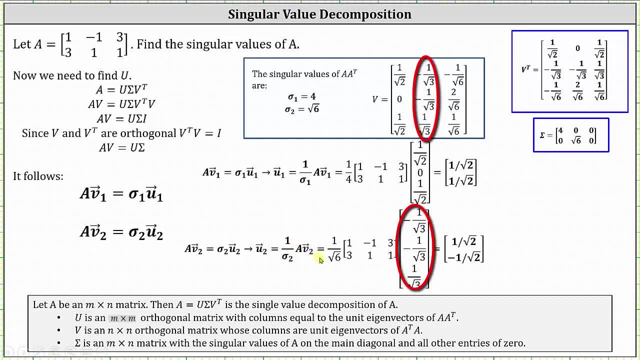 times matrix A times vector V sub two, which, again, I've already written out. The result is the vector U sub two, which has components: one divided by square root two negative one divided by square root two. And this is what we need to find: the matrix U. 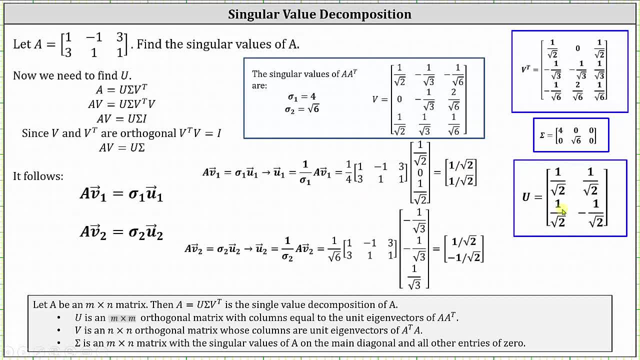 These two vectors form the columns of matrix U which we have here Now. you might be asking: why do we use these formulas rather than find the unit eigenvectors of A times A transpose? Well, remember, when it comes to these unit eigenvectors, 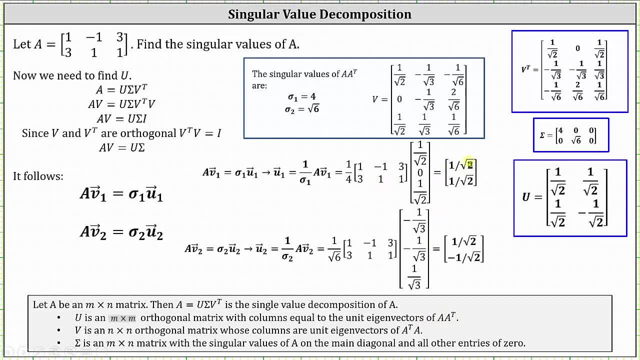 the first formula gave us vector U sub one equal to one divided by square root two, one divided by square root two. But there's also a unit vector in the opposite direction which, if we used, would not give us an accurate singular value: decomposition. 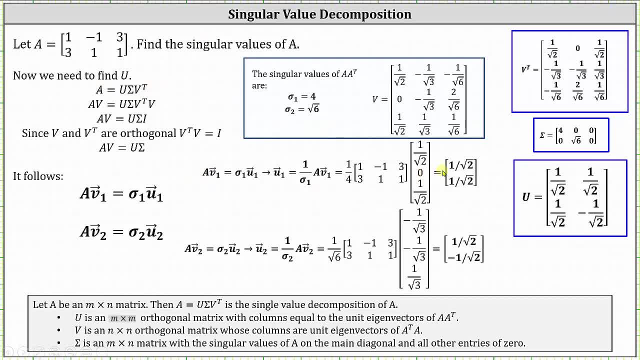 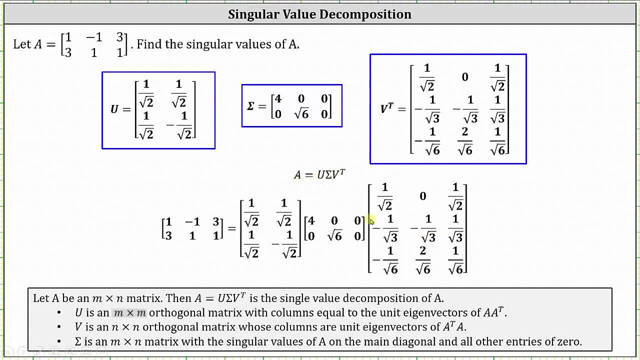 But by using the formulas we will get the correct unit eigenvector. So to finish this off, we now know A is equal to U times sigma, times V transpose, which I've written out here, which I also checked using the Desmos matrix calculator. 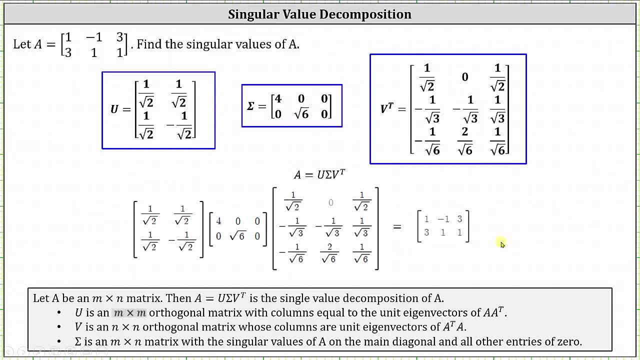 and the product on the right is equal to matrix A. I hope you found this helpful.